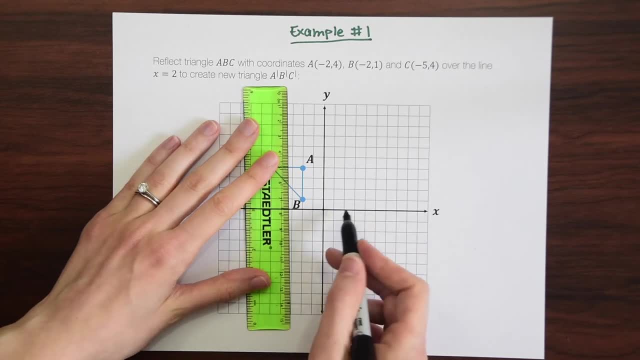 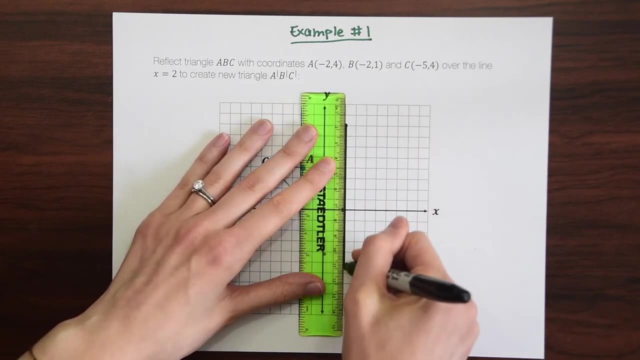 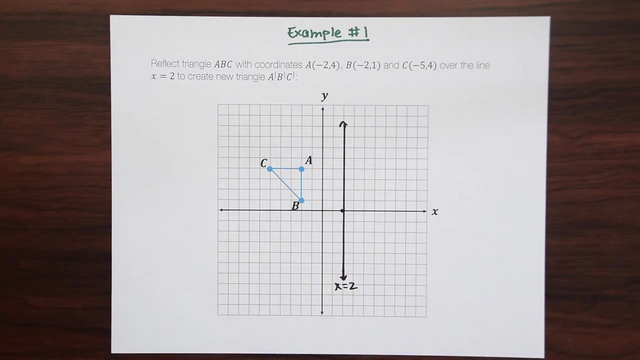 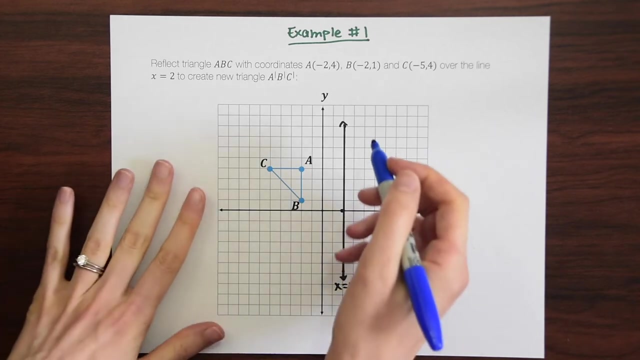 find x equals 2 on our x-axis here. so 1, 2.. So that's right here, And then we're just going to draw a line going down this entire thing. So let's leave it. x equals 2.. So now all we have to do is reflect each coordinate point one by one to the other side. 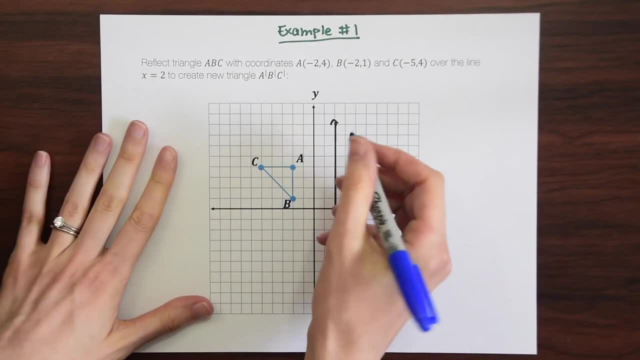 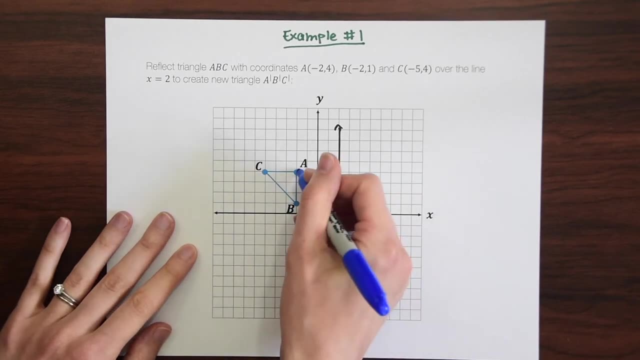 of this line. So we're making a mirror image and we want to measure out how many units away each point is. So if we look at point a, we can see it's 1,, 2,, 3,, 4 units away right: 1, 2, 3,. 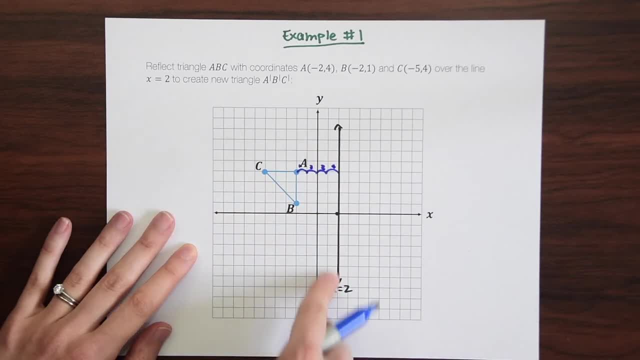 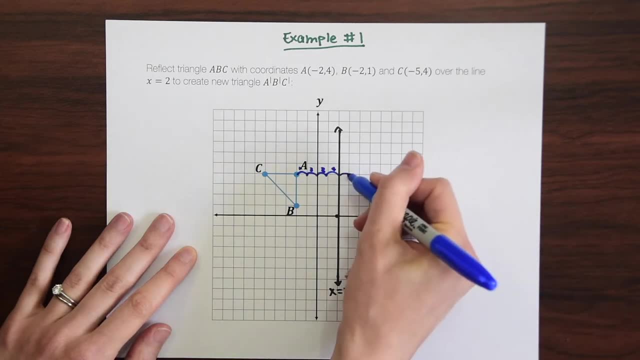 4 units away from our line. x equals 2, our reflection, And that's that line. And now all we want to do to reflect point a is to count 4 units on the other side of this line. So 1, 2,, 3, 4.. 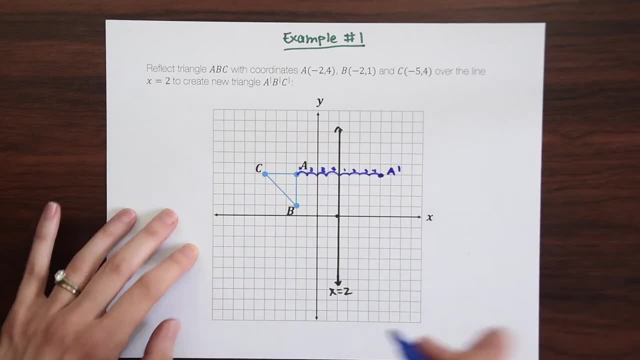 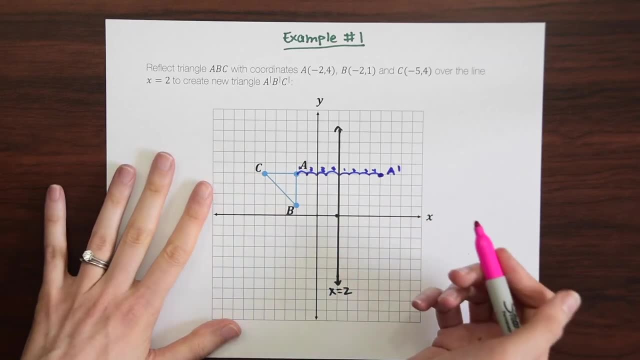 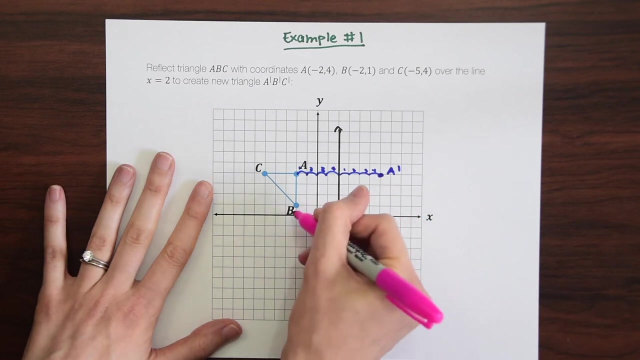 And this is going to be our new point a, prime. So let's just do that with each point I'm gonna- I'm just gonna use different colors here so we can see, to see easily what we're working with. So again, looking at point b, we have, we are 4 units away from this. 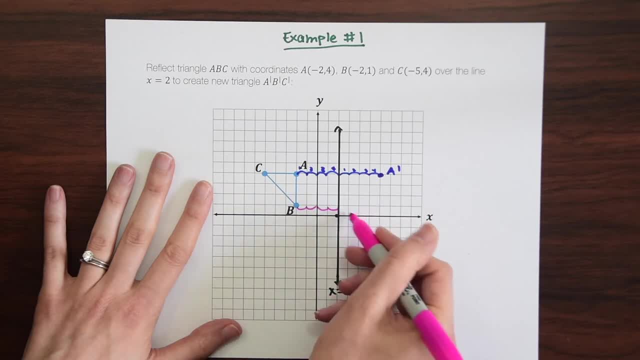 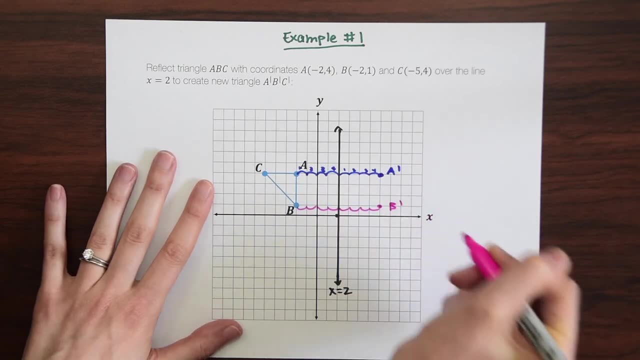 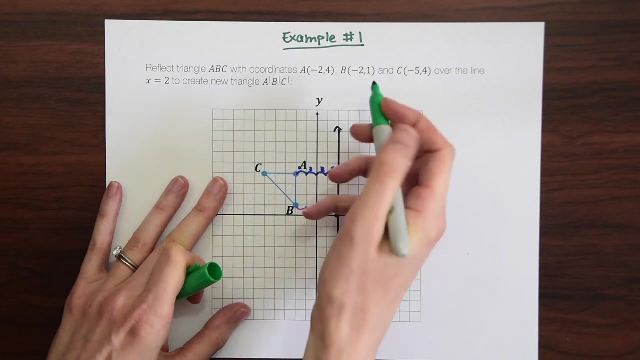 like one, two, three, four. and now we're just going to count four units to the other side of this line: one, two, three, four. and here we have our b prime. and lastly we have c. i'm going to measure up here just so we can see it more clearly. so c- let's measure the distance between c and line x- equals. 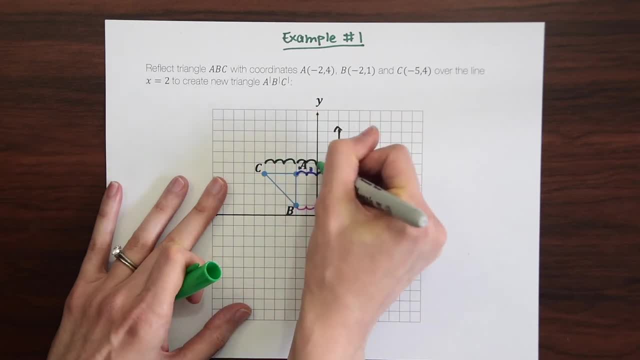 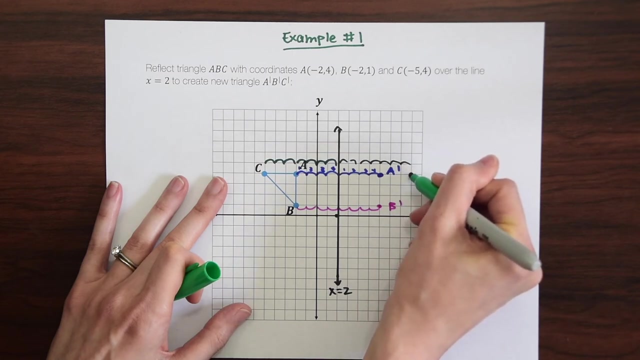 two. so we have one, two, three, four, five, six, seven. so that's seven units away from line x equals two. so now we gotta go seven units on the other side: one, two, three, four, five, six, seven, and we're gonna put a dot and then we can connect our dots. so our new triangle: a, prime, b prime, c prime. 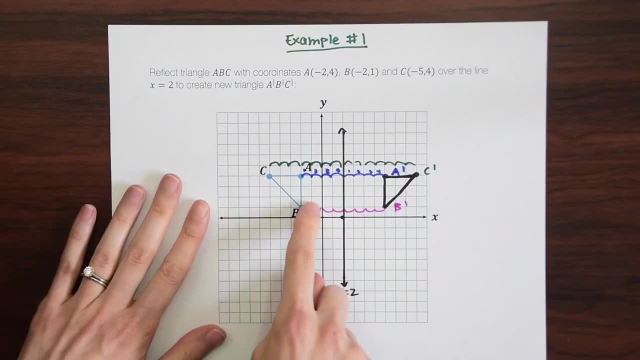 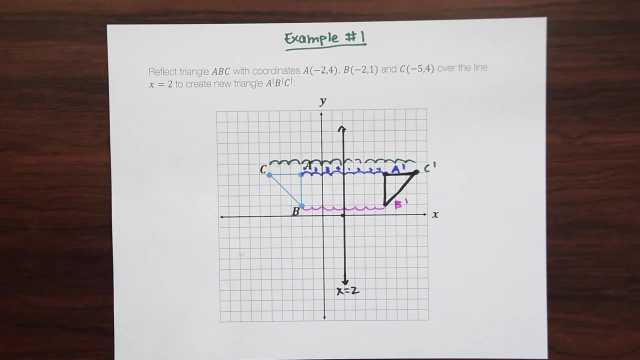 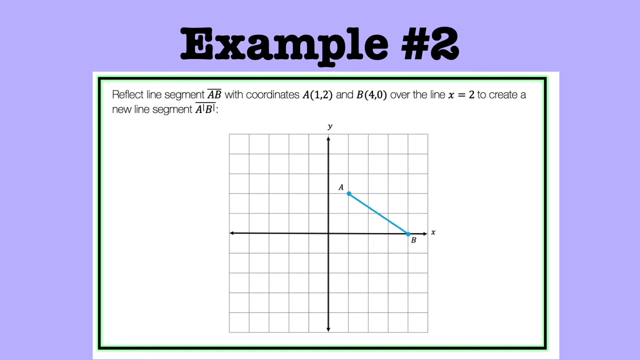 is is right here. so you could see that we reflected our image. each point is perfectly a mirror image away, equidistant away from this. line x equals 2 and that's our answer. so now let's look at another example. reflect line segment AB with coordinates a 1 comma 2 and b 4: 0 over the line x equals 2 to. 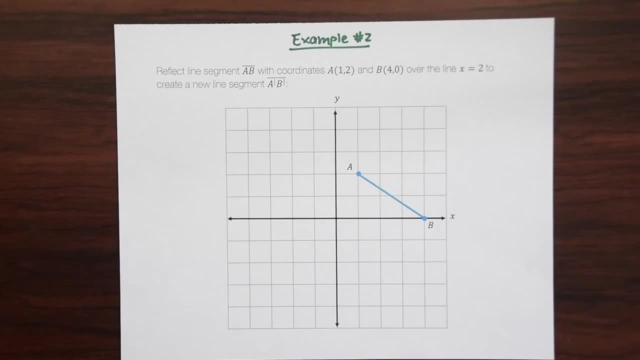 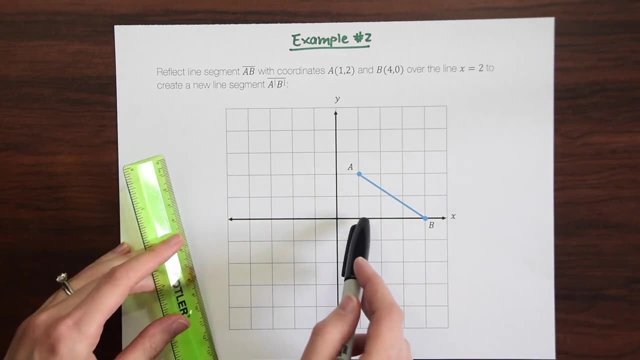 create a new line segment, a prime, B prime. so this time we're dealing with a line segment instead of a triangle. so again, let's draw out our line: x equals 2, so we go to where x is equal to 2, right 1, 2. so that's right here. and then we're 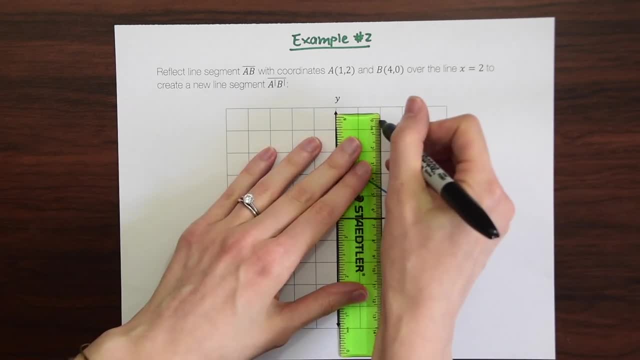 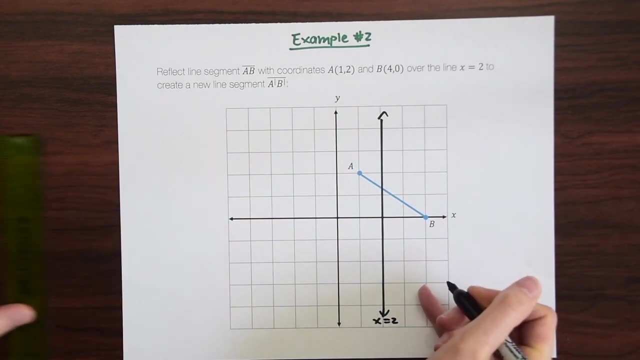 just going to draw a vertical line and label it: x equals 2. I know we can. we can take the mirror image of this point by point. so we only have two points. so this won't be so bad. but it's interesting because- notice- this is kind of being 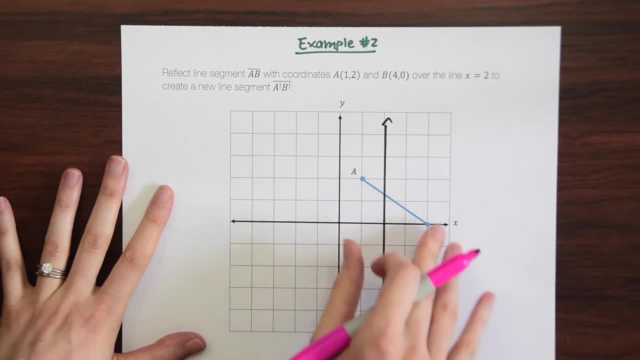 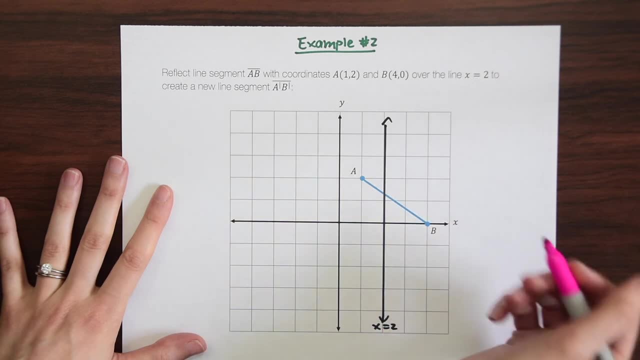 reflective of the line segment. so we're just going to draw a vertical line and reflect it onto itself, right? because we have a point here on one side of our reflection line and then we have another point B over here on the other side. so, but we're going to do this is the same exact way. so if you look, if you notice, 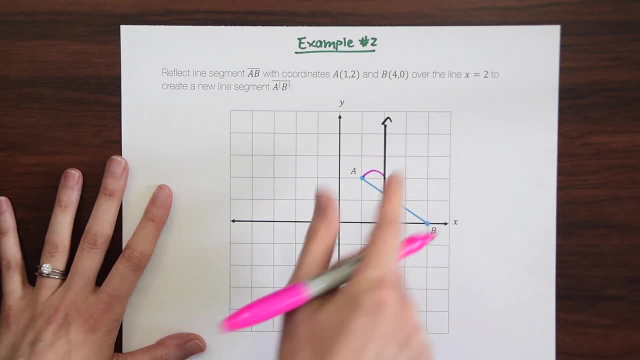 point a is one unit away from x equals 2, so we're just going to go one unit away from x equals 2- the other side. so this gives us a prime. and point B is two units away. it's not going to be from the line x equals 2, it's on the other side, but it's. 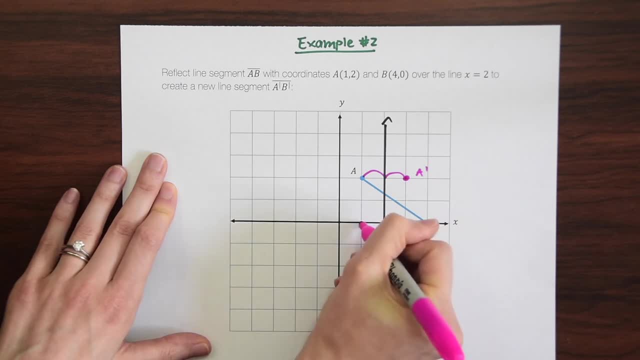 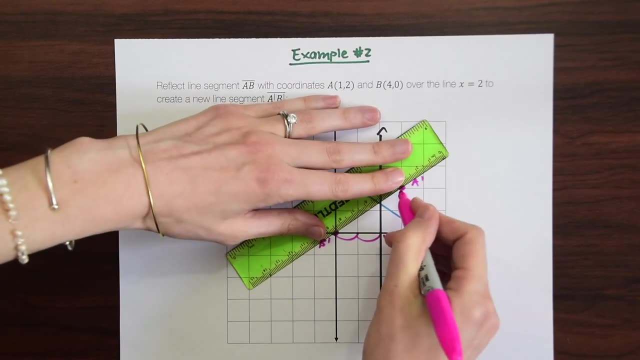 still two units away. so now we're just going to reflect that and bring it to the other side and label it B prime, and now we just need to connect our dots and you can see that this truly is in their image of itself, even though they are on. 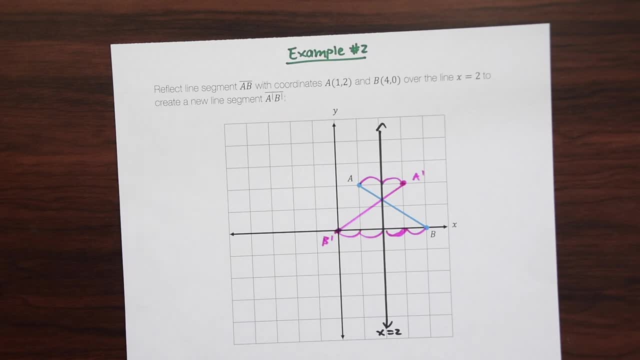 top of each other, like that, which is interesting, and the same would work for a more complicated shape like a triangle or Pentagon. any shape you're working with that's on to itself. you do the same exact thing. So if you're looking for more, check out the practice questions. 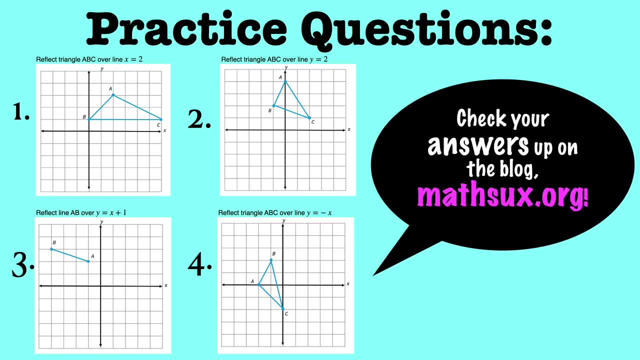 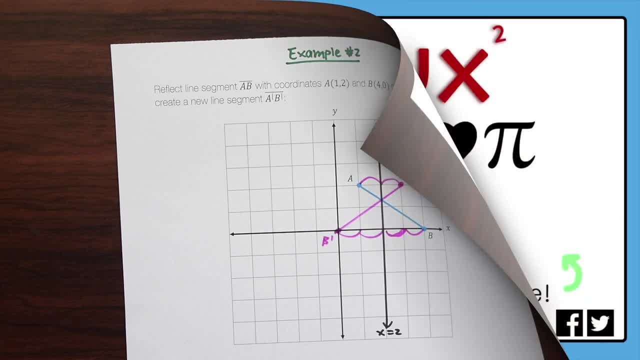 right here. The answers are up on my website, mathsucksorg. The link is in the description below And if you like this video, please give it a like and subscribe. Thanks so much for stopping by and happy calculating. Need more practice? Check out mathsucksorg for. 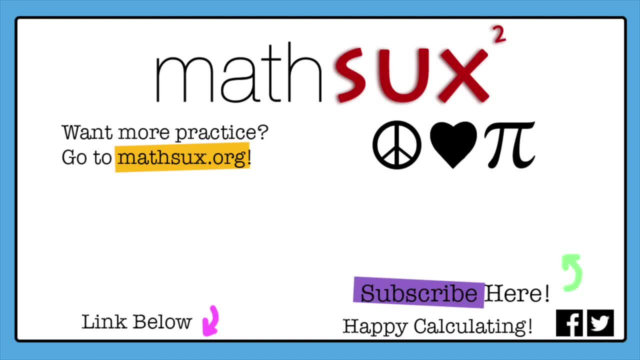 more questions: Link below. Also, don't forget to subscribe. Happy calculating.